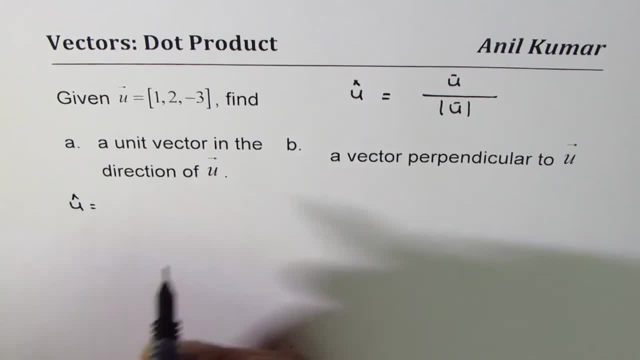 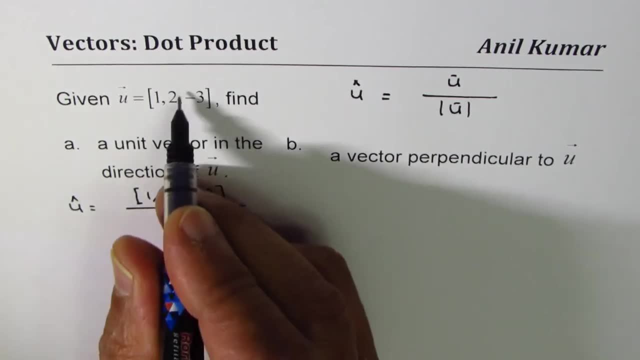 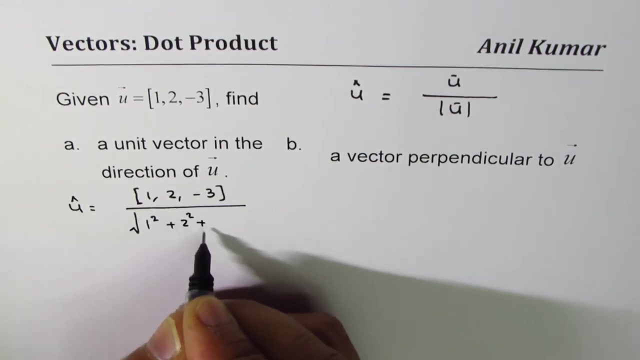 vector u. So unit vector will be the vector which is 1, 2, minus 3 divided by the magnitude. Magnitude of this vector is square root: 1 square plus 2 square plus minus 3 square. That is how you find the unit vector which is 1, 2, minus 3 divided by square root of 1 plus 4 plus 9.. 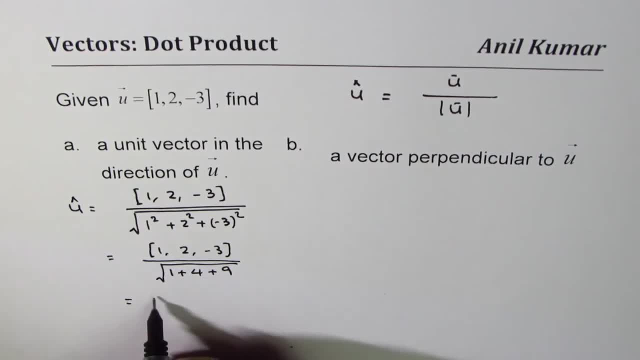 So which is 14? right? So 1 over square root of 14 times square root of 2.. 1, 2 minus 3, is it okay? or I should write this as 1 over square root of 14, 2 over square root of 14 minus 3 over square root of 14, so that becomes the unit. 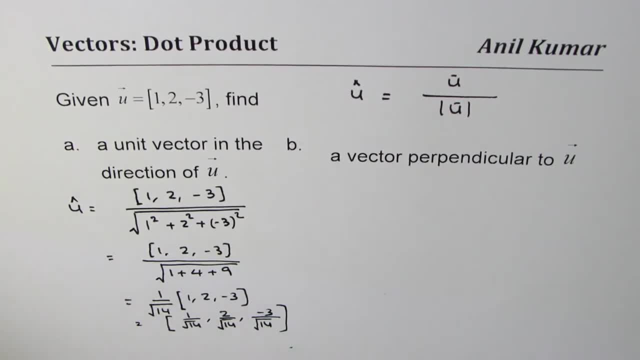 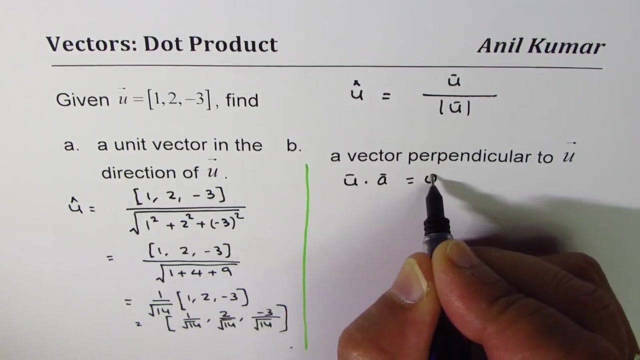 vector u. I hope the steps are absolutely clear, right? so that's how you find unit vector. now let's do part B, which is a vector perpendicular to you. now let's consider a to be perpendicular to V. U then dot product of vector and you should be equal to zero if you is perpendicular to vector a. correct the. 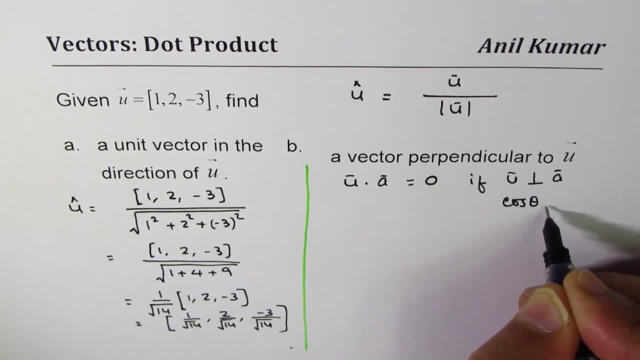 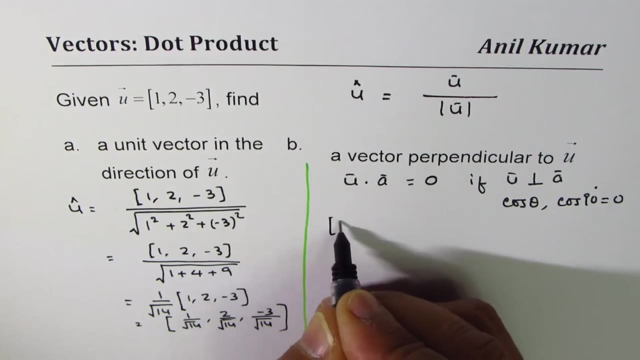 reason is cos theta, which will be in this context, and that is the northbound surface of this vector. so this is a case: cos of 90 degrees becomes 0, right, That's the whole idea. We don't know what A is, but we could write this as the dot product, as 1,, 2, oh, I mean, I want to write. 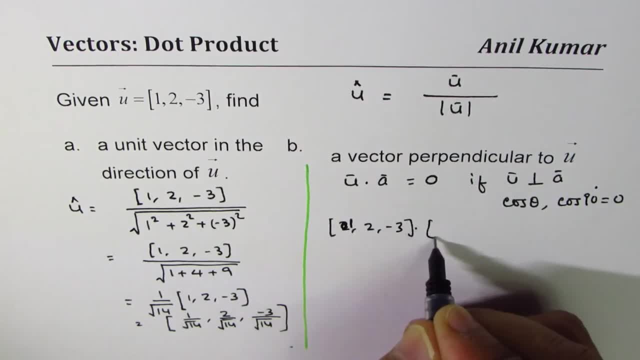 1, let me write 1,, 2, minus 3, dot the components P, A1,, A2, A3. So this is equal to A1 times 1, so it's A1, plus 2A2, minus 3A3, and that should be equated to. so this implies this: 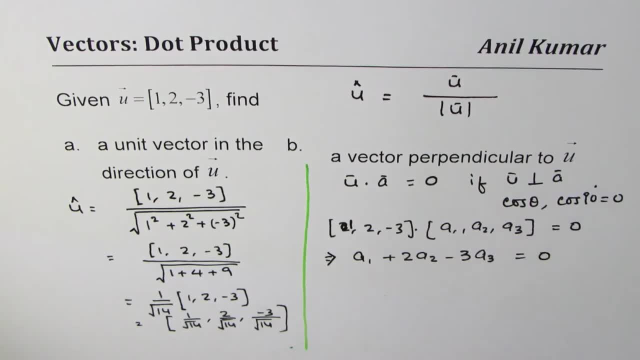 and we have to equate this to 0, right, So it equals to 0.. So any combination of these A components resulting into a 0 will give us the dot product. So in R3, we could have many components.